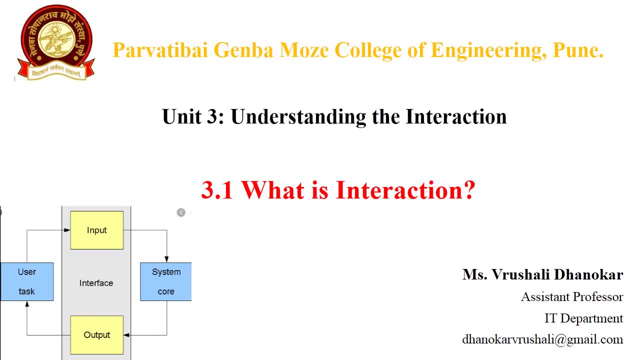 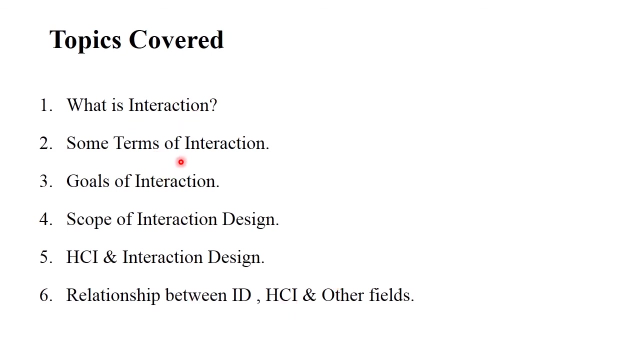 So what is mean by Interaction? What is the goal of Interaction? Ok, So this video covered Interaction related each and every points. Ok, So let's see what is mean by Interaction Next. So these topics are covered in this video. that is what is Interaction, some terms of Interaction, Goals of Interaction, Scope of Interaction Design. then Human-Computer Interaction and Interaction Design, and Relationship between Interaction Design, Human-Computer Interaction and Interaction Design. 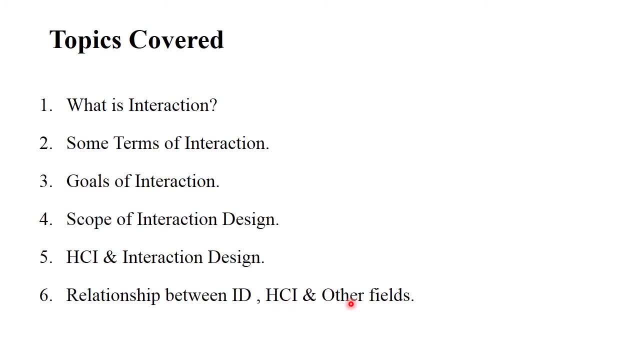 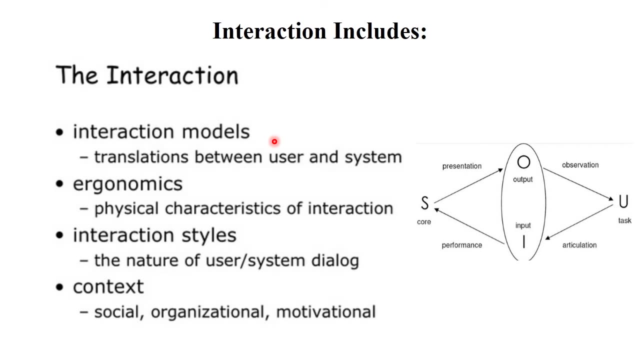 Ok, Delete Neutral. so some basic of things And next So butterfly. The point is to getdon normal connection data at all points. Yes, situations and factors are also related to Interaction, merged with subject function andلام, Human-Computer Interaction and other fields. 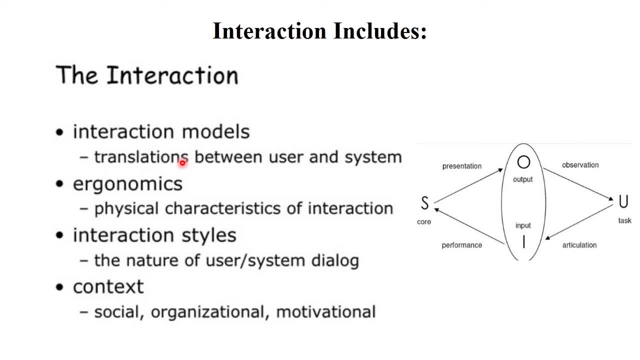 Ok, All topics are covered in this video, So let's see one by one how exactly it works. Ok, So interaction includes: Ok, This is the summary of this unit regarding information. okay, unit 3 also contains about: contain about ergonomics. 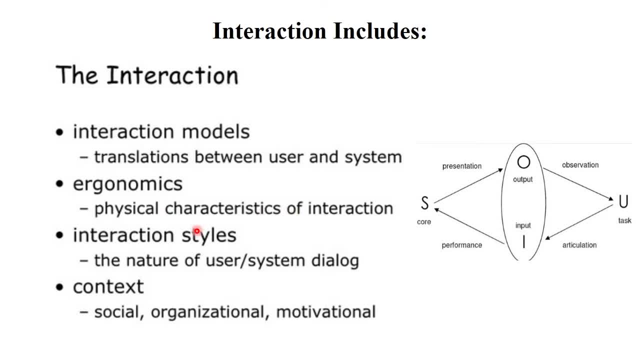 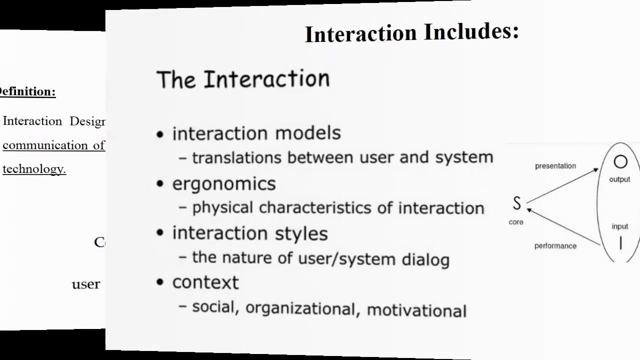 ergonomics means physical characteristics of interaction, then interaction styles, the nature of user and system dialogue, and also different context, that is, social, organizational and motivational. okay, so we will see these all points one by one in my next video. okay, this video contains only about interaction. what exactly it means? okay, next, 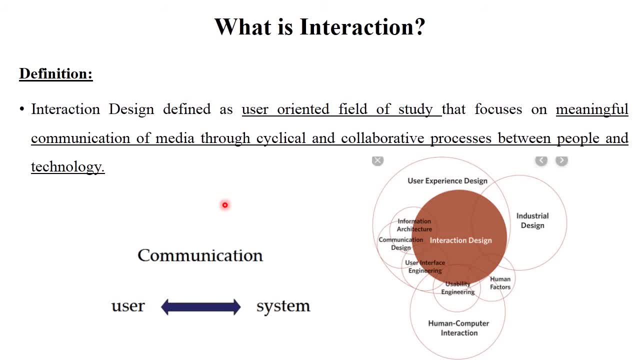 what is interaction? so interaction simply means communication between user and system. clear communication between user and system, okay, but the definition of interaction is: interaction is as user-oriented field of study, that is, focus on meaningful communication of media through cyclical and collaborative communication of media through cyclical and collaborative. 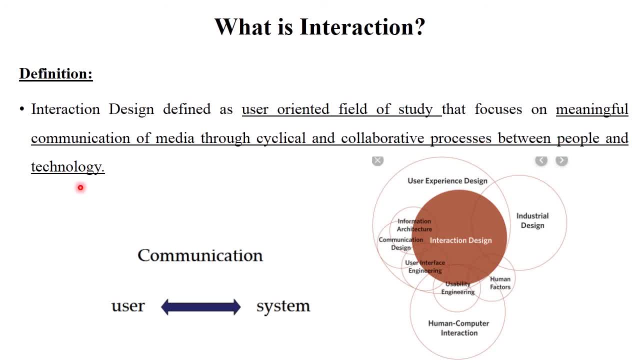 process between people and technology. okay, this is the definition of interaction. it is the cyclical and collaborative process between people and technology. okay, so interaction simply means communication between user and system, communication between different people with different technologies. clear, so interaction design: see here. interaction design is common in each and. 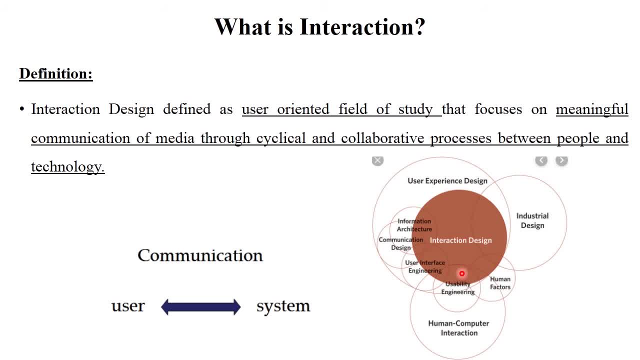 every field. okay, each an every field. computers are used. people's interact with computers by some different purpose or different requirements. right so interaction design is is in between user experience design. it also involve industrial design, Usability engineering, human factors, information architectures, communication design and human computer interactions. okay so, each and every. 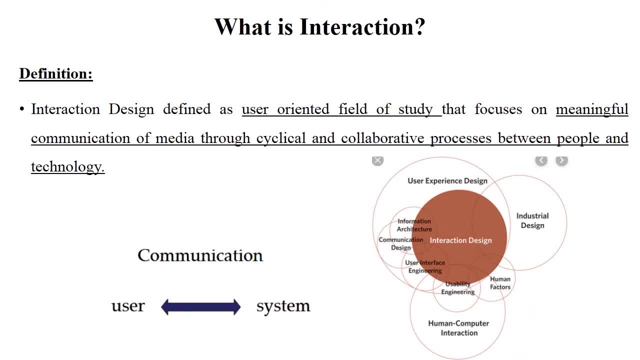 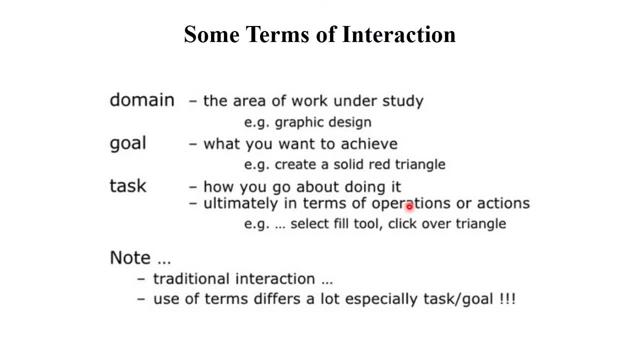 field use, interaction design clear. Next, Now, there are some terms of interactions. Which terms are included in interaction? There are total three terms, that is, domain, goal and task. So what is mean by domain? So domain means the area of work under the study, For example graphics design. Graphics design is one domain. 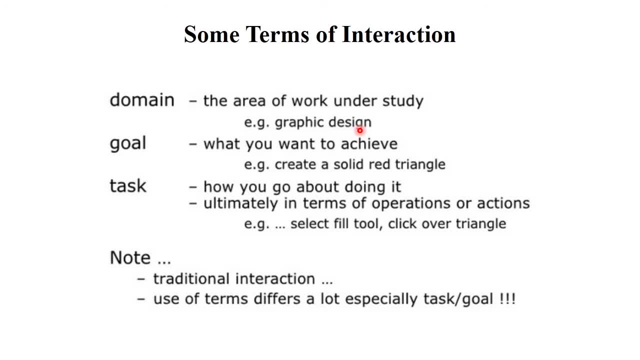 or we can say domain also. we consider as one organization, one department, etc. Okay, now next one is goal. What is mean by goal, What you want to achieve? Okay, what is your aim? This called as goal, For example, in graphic design domain, the goal is create a solid red. 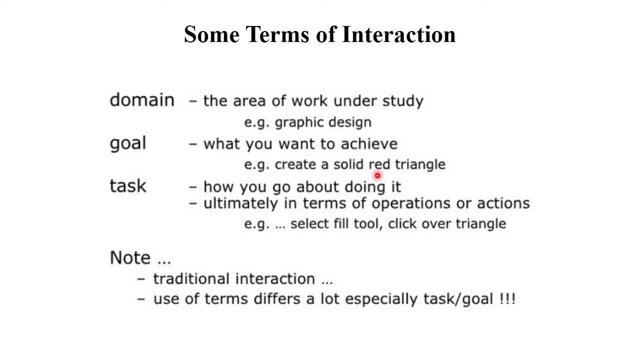 triangle. Okay, this is the design You need to create solid red triangle. This is your goal. Clear, And the next term of interaction is task- How you go about doing it Ultimately in terms of operations or actions. Okay, your goal is create a solid red triangle. Okay, now what you 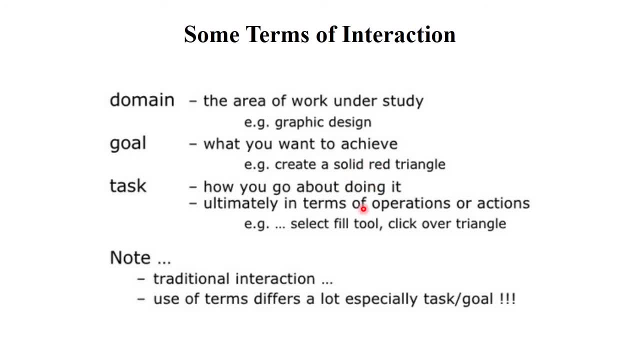 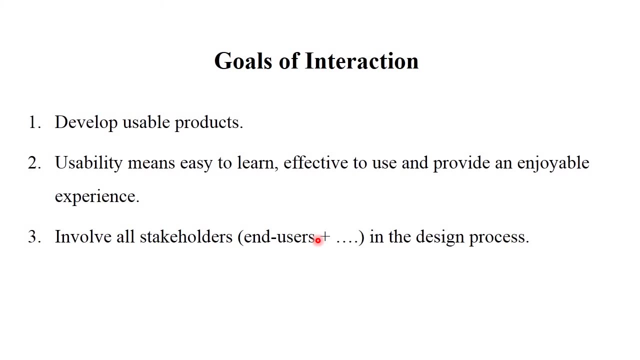 perform for that, for accomplishing this goal: Select, fill, tool, click over triangle, etc. Clear. So these are the terms which includes in interaction: domain, goal and task. Clear. Okay, next Now goals of interaction. The main goal of interaction is to develop a usable 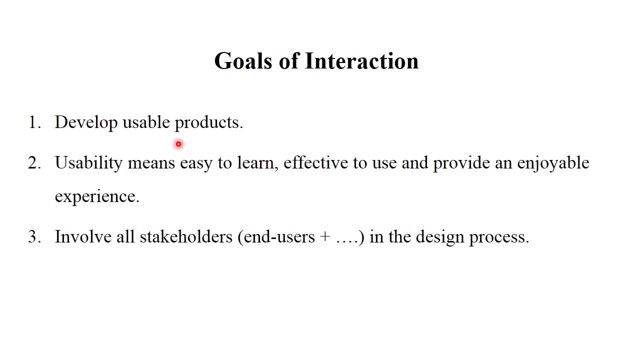 product: Okay, we use different types of products or different types of applications. For example, we all are used mobile- Okay, we use only that application that are more interactive. different types of social media applications like WhatsApp, Facebook, then Insta, Right, This all types of 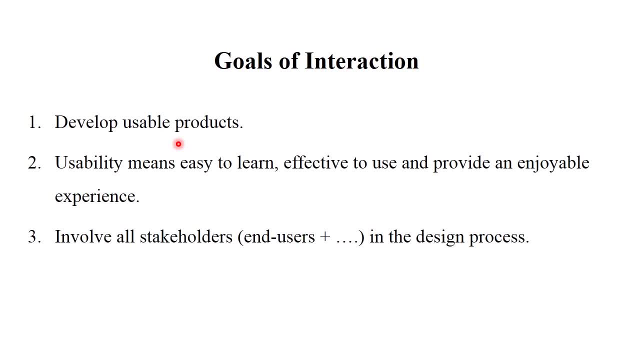 application we used because these are more interactive or attractive, purpose Right. And also there are different payment app like phone pay, ATM. Then there are also different online services app like Flipkart, Amazon, Clear. So we use only usable products. Clear. Then, what is meant by usability? Okay, I already told you, usability means easy to 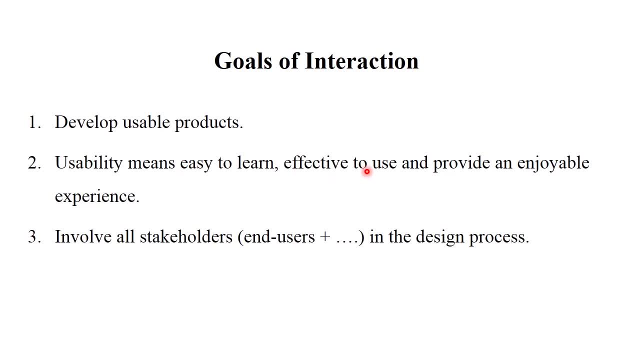 learn and easy to use. It is effective to use and provide an enjoyable experiences. Okay, So goal of interaction involves all stack holders, end users, etc. in the design process. so what is mean by stack holder? see here when you will develop a particular product. ok, so designer. 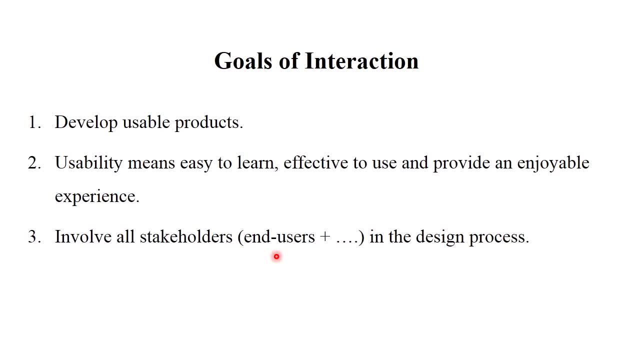 then customer, then their developer. ok, then their planning and requirements persons, testers- this all types of persons involved in that product- ok, and this- all types of persons- is called as stack holders. ok, so stack holders means the persons which involve in the start to end process of that particular product. clear, so this is the goal of interaction, ok, next now scope of 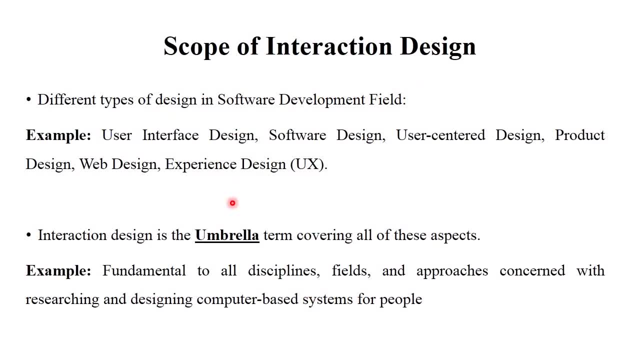 interaction design. ok, we all are familiar with this scope of interaction design, or in which field this interaction designs are work. ok, different types of design used in software development field, that is, user interface design, software design. then also there are user centered design, product design, web design, experience design and other design tools, like you will see. 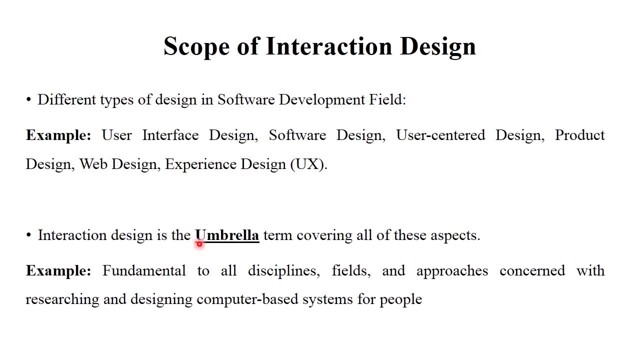 etc. Okay Now, interaction design is the umbrella term, covering all the aspects. Okay, What is mean the umbrella term? Umbrella term simply means interaction design used each and every field or each and every aspects. Clear Interaction design is used, fundamentals to all disciplines. 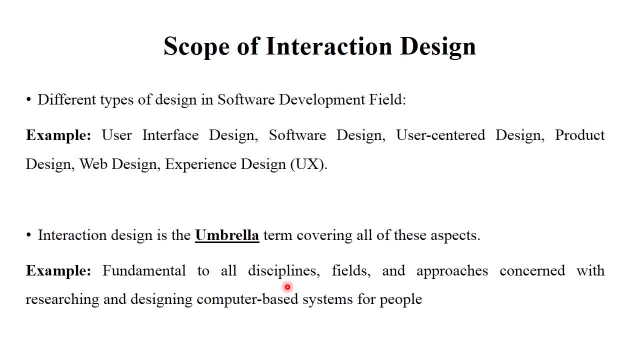 or all areas, whether it is technical area or whether it is non-technical area. Interaction design also used in different fields and approaches concerned with researchers designing computer based systems of peoples, etc. Clear. So these are the scope of interaction design. Of course, interaction have wide scope. Clear, Okay. Next. 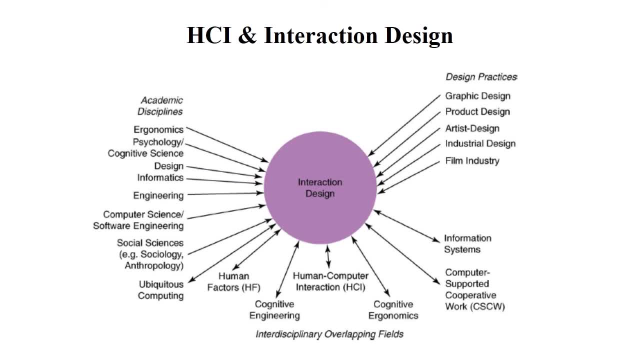 An interaction design. Human computer interaction is one field of interaction design. Okay, Interaction design involves: see here: There are different types of interaction design. There are different types of interaction design. There are different types of interaction design. There are different types of design practices like graphic design, product design, artist. 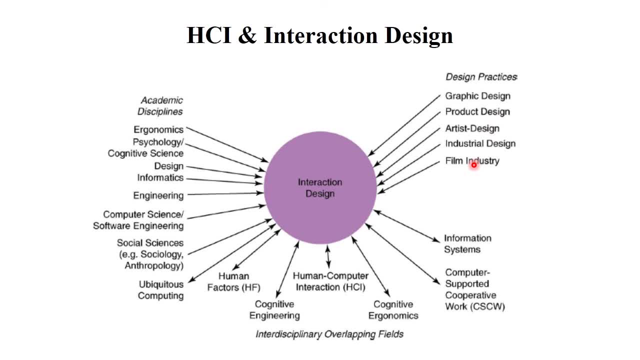 design, industrial design In film industry also. interaction design or computer interactions are work. Okay. Also there are some information systems, Computer supported cooperative works. Also cognitive ergonomics, human, computer interaction Clear. So this arrow between two words, both meant to or one to one relation Clear Now: cognitive engineering and human. 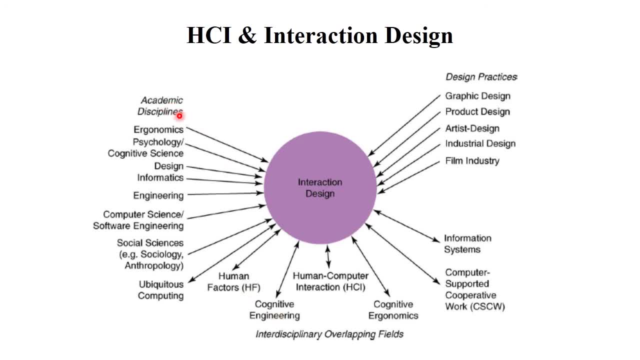 factors: Okay, Also, interaction design, useful in academic disciplines. Ergonomics: What is meant by ergonomics I will explain in my next video. Okay, Then psychology, cognitive science, design, informatics, engineering- Okay, Engineering is one of the familiar term where computer centers are used. 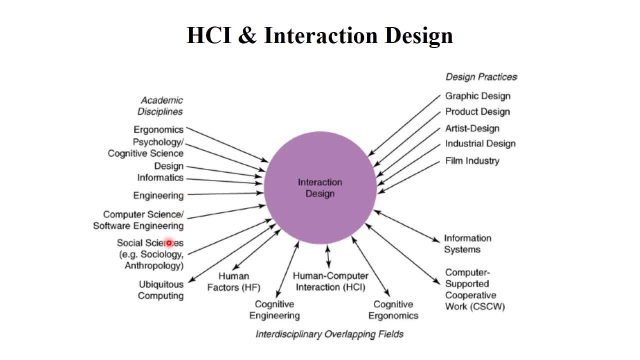 Okay, Then computer science and software engineering, Social science- Social science includes sociology and anthropology- Then ubiquitous computing. Clear So each and every field or each and every term there is human computer interaction and interaction, designs are used. Clear This. 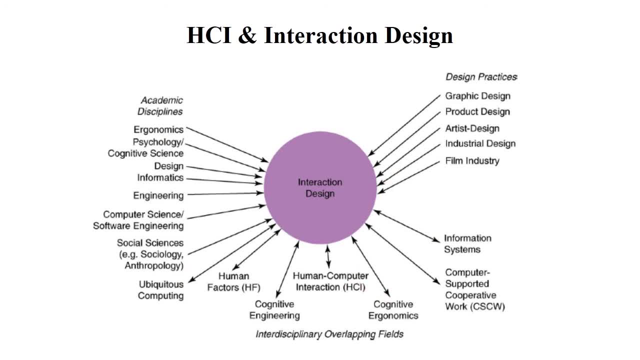 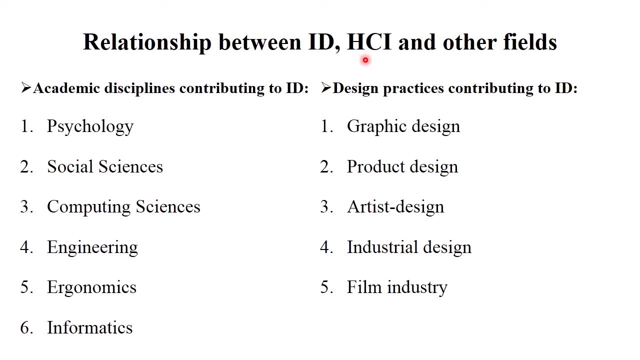 is the interdisciplinary fields of interaction design: Okay. Next, Relationship between interaction design, human, computer interaction and other fields: Okay. So see here These are academic disciplines contributing to interaction design: Okay. Academic disciplines means study approach: Okay. Or educational field. 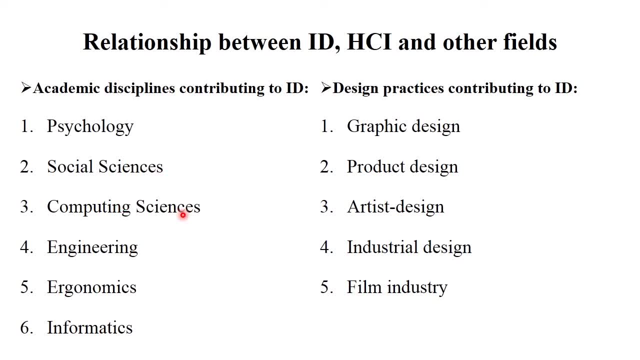 Like psychology, social science, computing science, engineering, ergonomics and informatics. This or academic discipline field interaction designs are used, Clear. And next there is design practices contributing to interaction design. Which type of design practices are used? There will be. 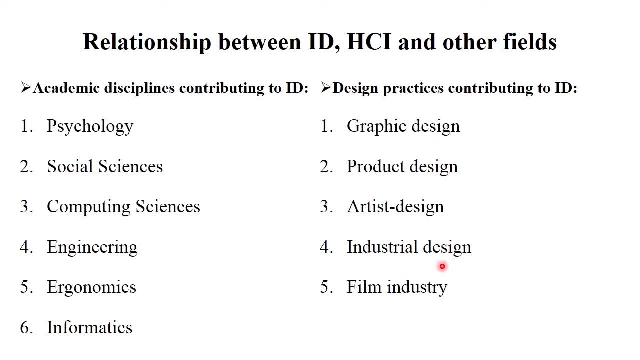 graphic design, product design, artist design, industrial design and film industry- Clear. In this way, each and every field- Interaction design and human computer interactions- are work Okay, And we know that how to work Okay. Next, relationship between, again, interaction design and human computer.